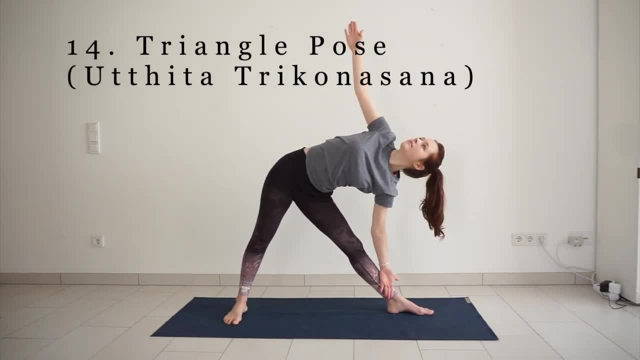 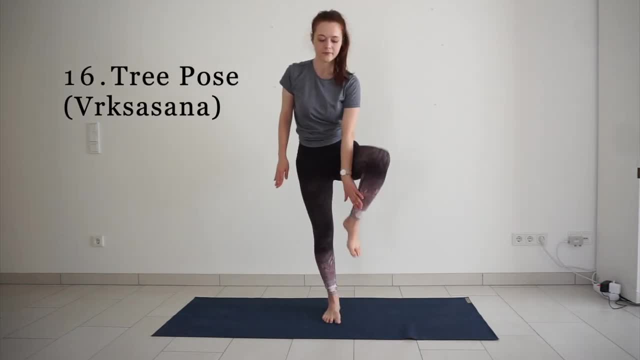 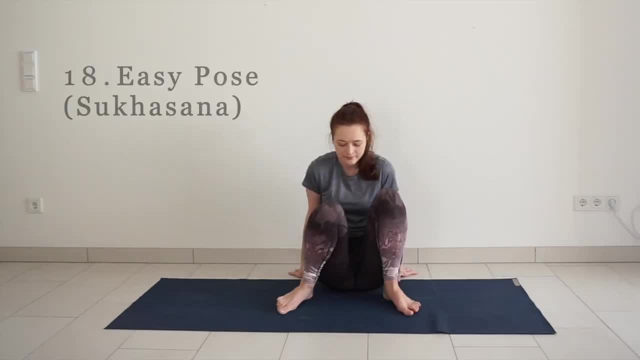 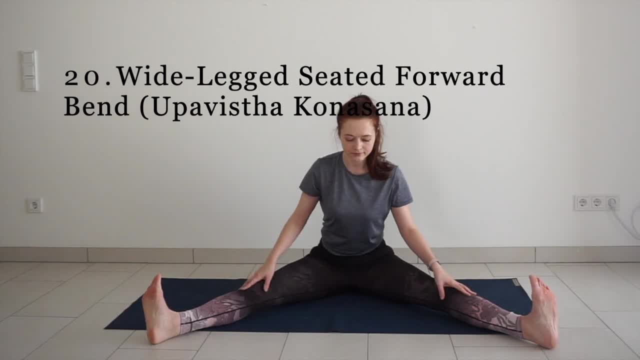 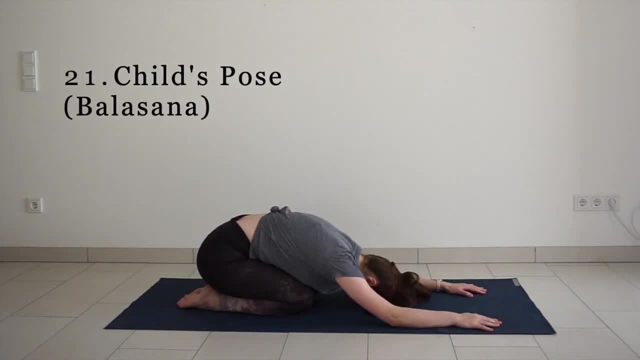 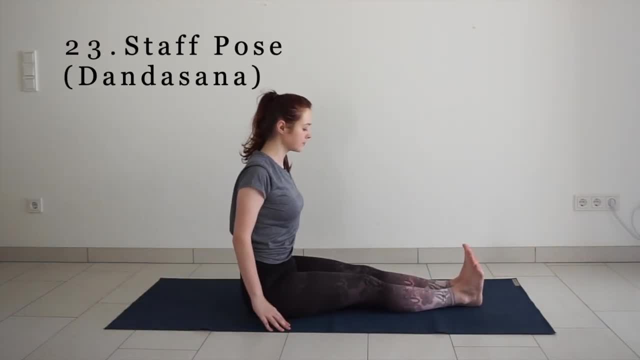 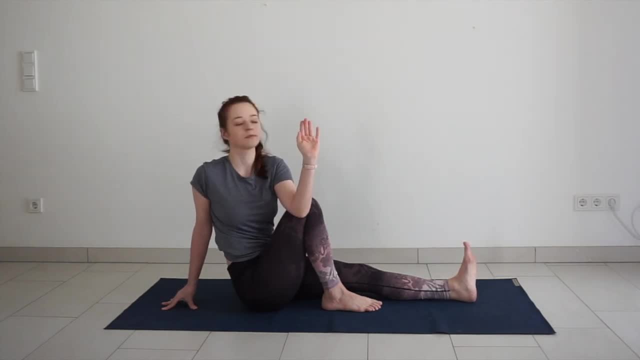 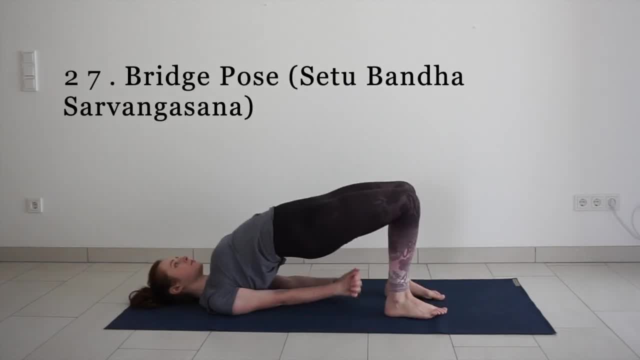 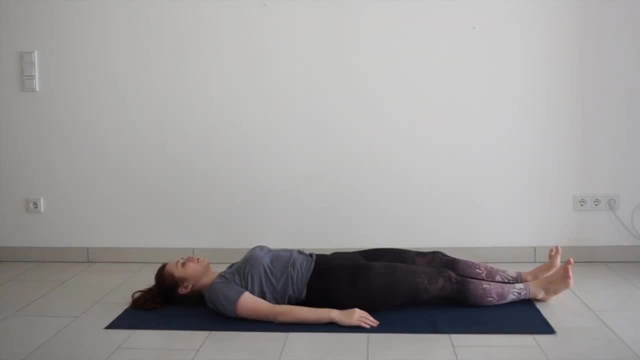 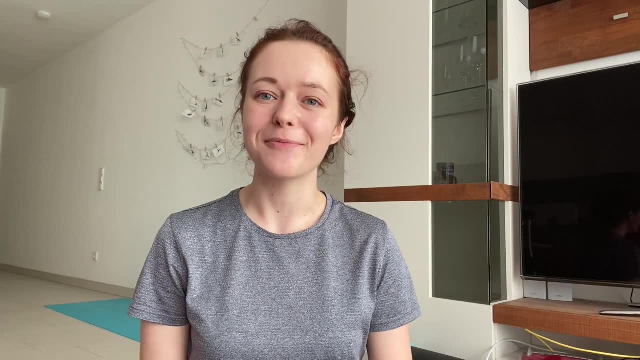 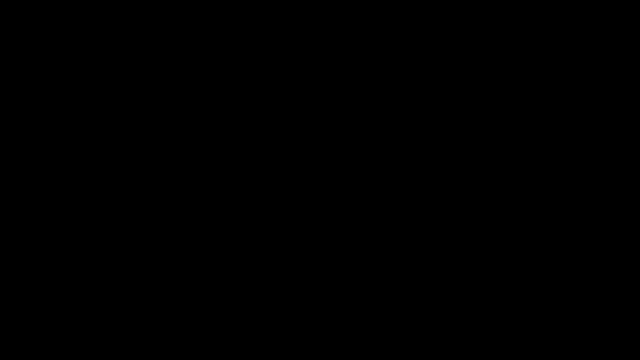 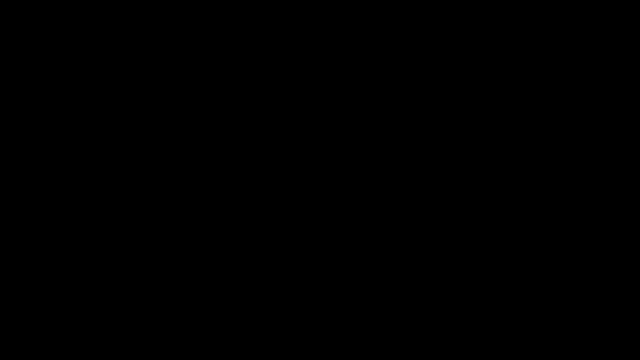 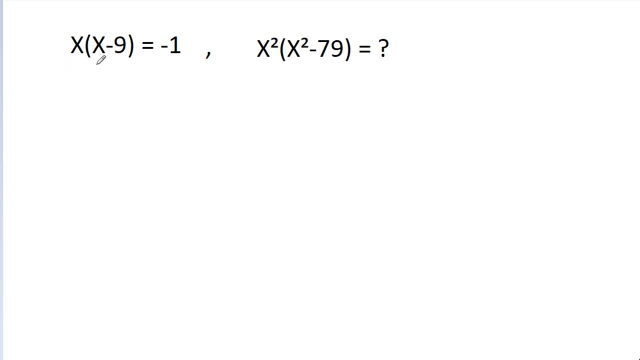 In this video we have given that x times x minus 9 is equal to minus 1.. Then we have to find the value of x square times x square minus 79. So we have x times x minus 9 is equal to minus 1.. That means x minus 9 will be equal to minus 1 by x, And it is x plus. 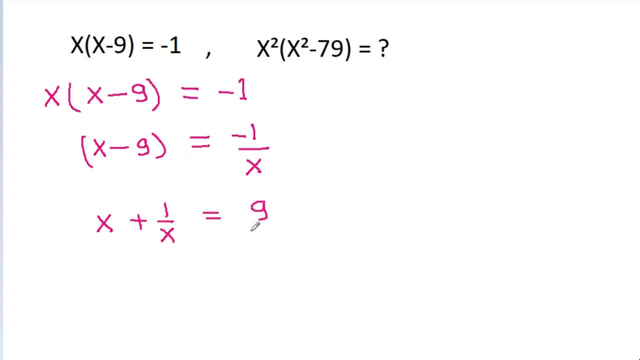 1 by x is equal to 9.. And if we square it both sides, then x plus 1 by x, whole square will be equal to 9 square, And it is x square minus 1 by x, square plus 2 times x times 1. 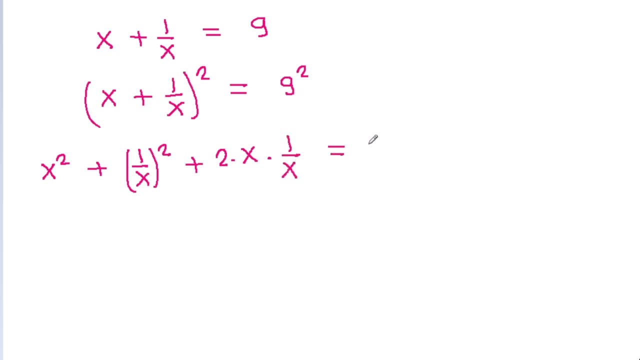 by x is equal to 9, square is 81. And x will get constant. So it is x square minus 1 by x square plus 2 is equal to 81. And x square plus 1 by x square will be equal to 81 minus. 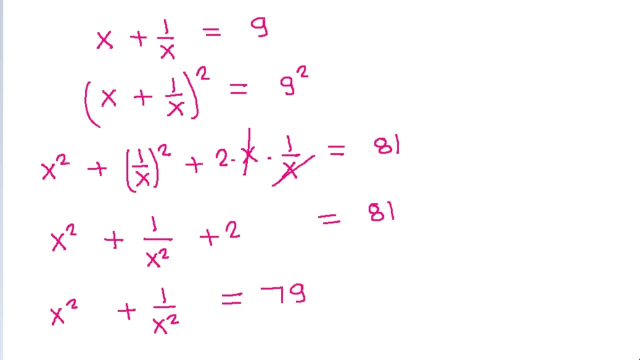 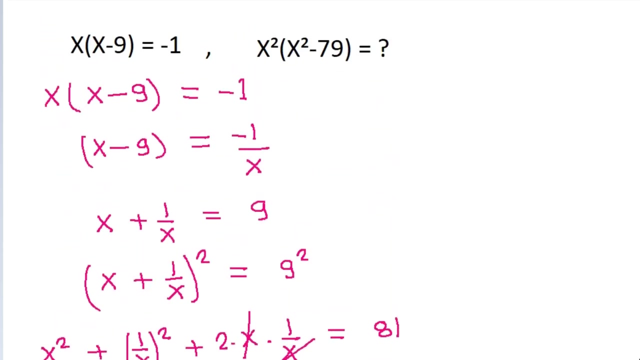 2 will be 79.. And it is x square minus 79 is equal to minus 1. by x square minus 2 is equal to minus 1.. So x square times x square minus 79 will be equal to minus 1. It is minus.